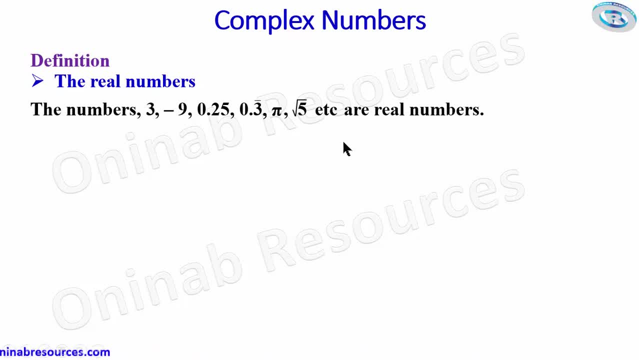 This is said to be the second largest set of numbers. Also, we look at the imaginary numbers. The numbers square root of negative 4, square root of negative 9, square root of negative 5, and so on give birth to another set of numbers. 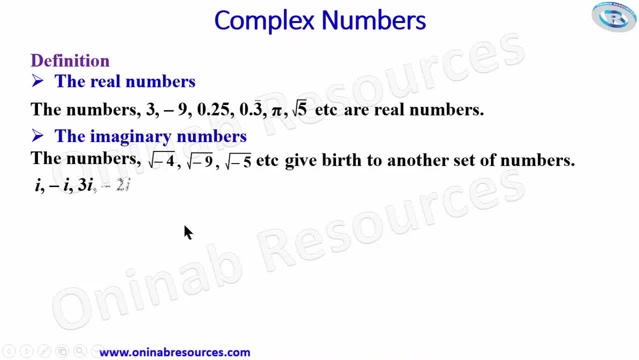 i, negative i 3, negative 2i and so on are called real numbers, The imaginary numbers. The fact that we cannot find the exact value of square root of negative 4, negative 9, or negative 5 by any mean, that gives birth to the set of number i, where i is square root of negative 1.. 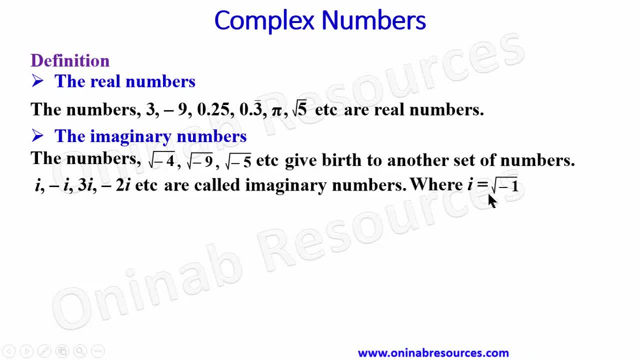 So, since we cannot find the exact value of square root of negative 1, we look at the imaginary numbers. So, since we cannot find the exact value of square root of negative 1, it is represented by i and this i is called imaginary number. 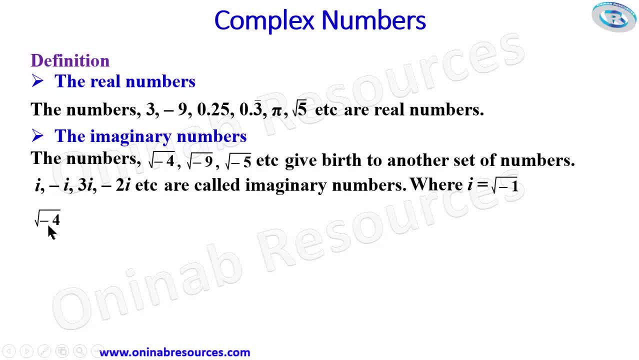 So that from here we can have square root of negative 4.. Since negative 4 can be written as 4 times negative 1, so we have it as square root of 4 times square root of negative 1.. And we want the square root of 4 to be plus or minus 2.. 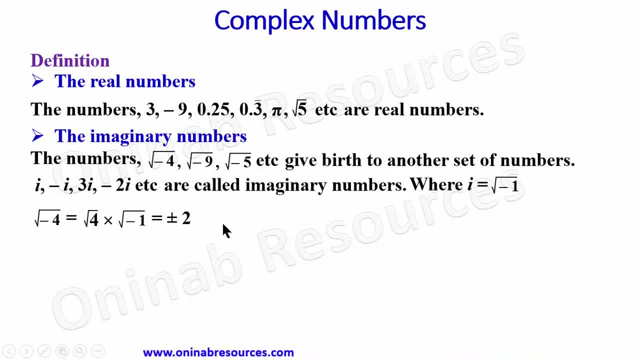 And this root of negative, Negative 1 is i. Here, this square root of negative. 9 can be written as positive or negative. 3i and so on. These are called the imaginary numbers, Then the complex numbers. The complex numbers is the largest set of numbers, because every real number can be written as complex number. 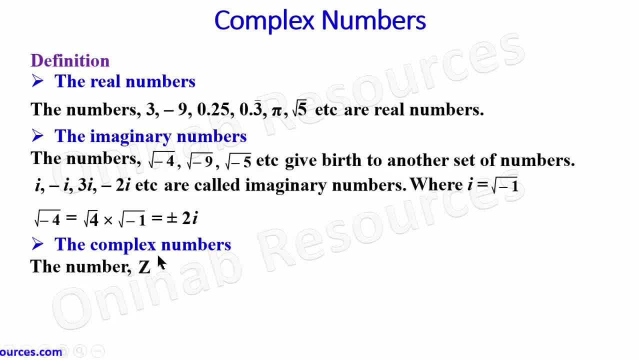 We now look at the definition. The number represented by z is equal to a plus b. i is called the complex number, where a is the real part and b? i is the imaginary part. So you can see the real number plus or minus the imaginary number give birth to the complex number. 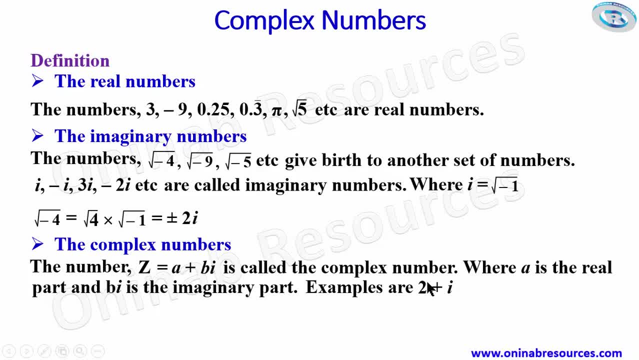 Examples are: We have 2 plus i, where 2 is the real number and i is the imaginary number. We have pi minus 3i, where pi is the real part and the 3i is the imaginary part, and so on. 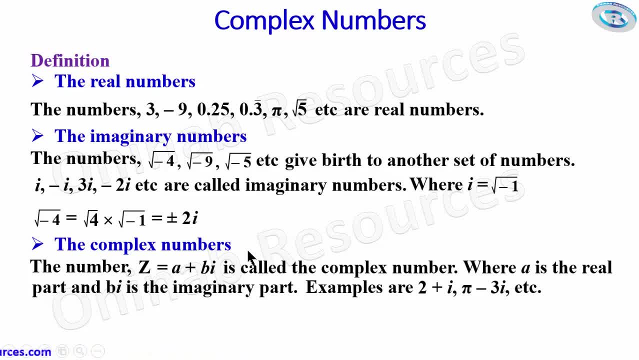 Like we said earlier, the complex number is the largest set of numbers. Like here now, if I have 2 plus 0.. I, which means it is 2.. That's real number, But the imaginary part is 0.. We can also have another complex number whose real part is 0.. 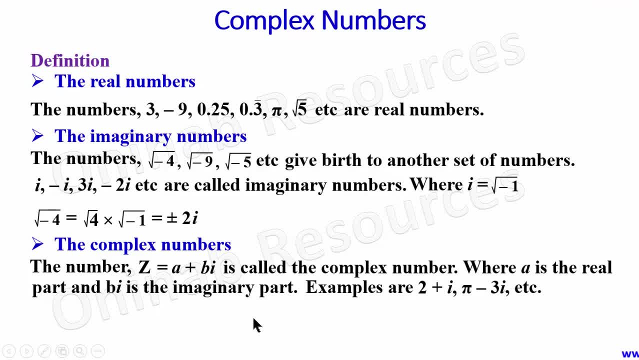 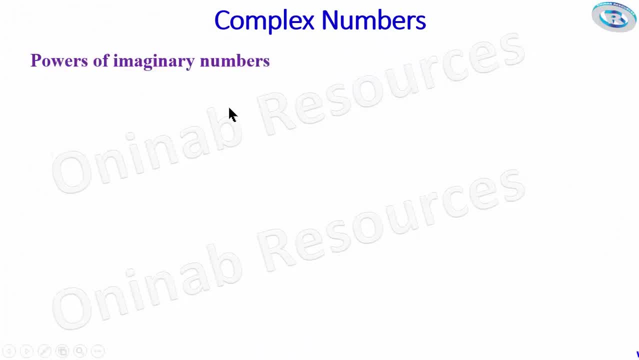 So these are what we are going to be looking at here Now. in our next slide we'll be looking at powers of imaginary numbers. So we have i raised to the power 7.. We have i raised to the power 2.. We know i is square root of negative 1.. 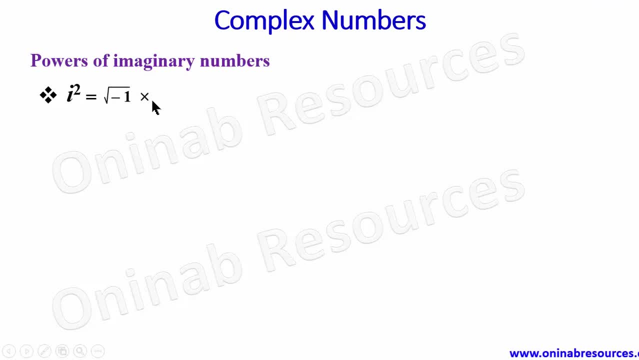 So i squared is square root of negative 1 times square root of negative 1.. And that will give us negative 1.. Then we now have i raised to the power 3.. This is i squared times i. So we know that i squared is negative 1.. 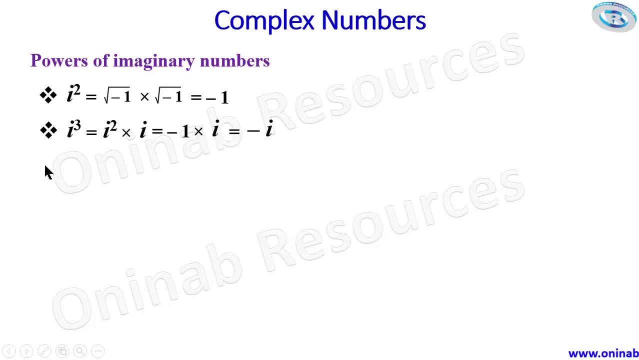 Then multiply by i And that gives negative i. Then also we have i raised to the power 4.. i raised to the power 4 can be split into i squared times i squared And we have i squared to be negative 1 times negative 1.. 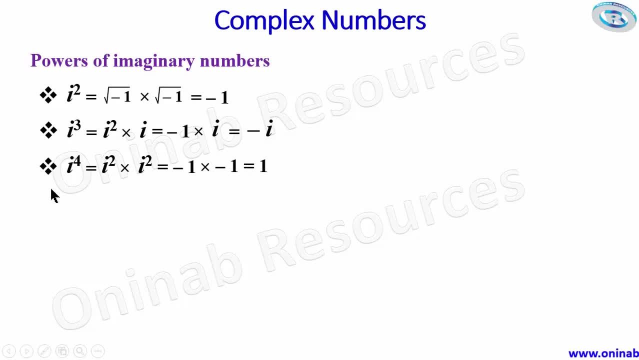 And that gives positive 1.. Then we look at: i raised to the power 5.. i raised to the power 5 is i raised to the power 4 times. i Remember our law of indices. This is i raised to the power 1.. 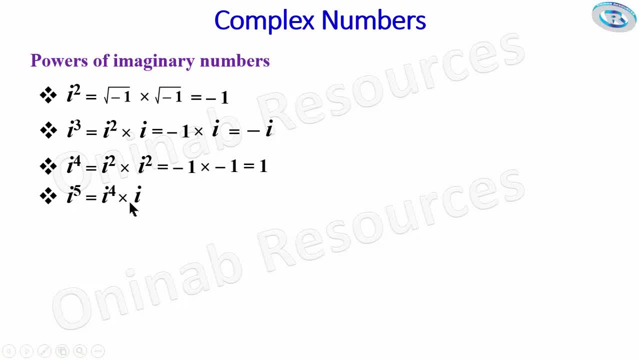 Since we are multiplying, we add. So i raised to the power 4 is positive. 1, then times i And that gives i. We now look at i raised to the power 15.. Now, how do we get this very large number? 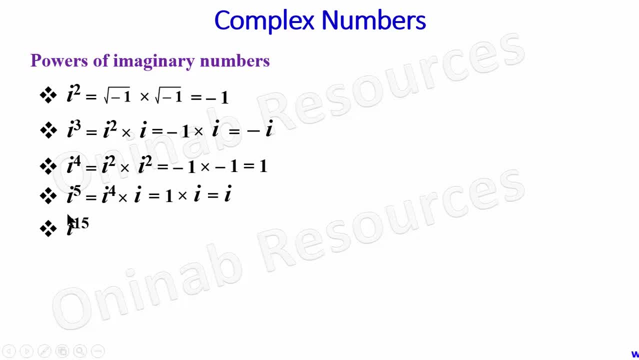 If we have a very large number like this, we divide 15 by 15.. When we divide 15 by 4, we are going to have 3 remainder 3.. Since we have 3 remainder 3, so the quotient is 3.. 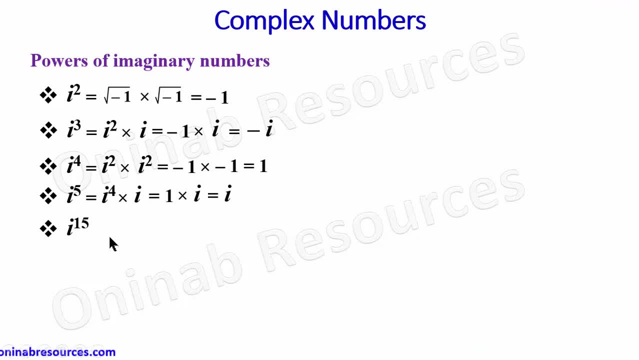 We multiply it by 4. It gives 12.. Then plus the 3.. Which means we can write: i raised to the power 15 as i raised to the power 12, then times i raised to the power 3.. Or we can just look for multiple of 4.. 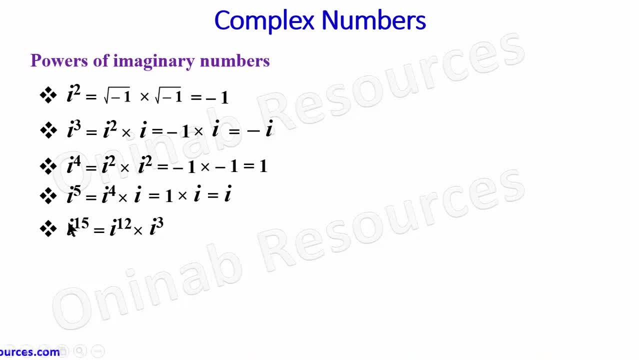 The largest multiple of 4 we can get from 15, which is 12.. And we then add 3 to make our 15.. We can then write this as power of 4.. That's going to give us: i raised to the power 4, then raised to the power 3.. 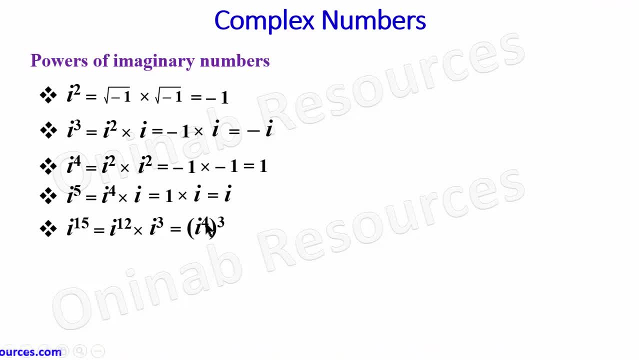 See applying law of indices. i raised to the power 4.. Then all to the power of 3. We just multiply the indices, Then times. i raised to the power 3. We just split this into this by application of law of indices. 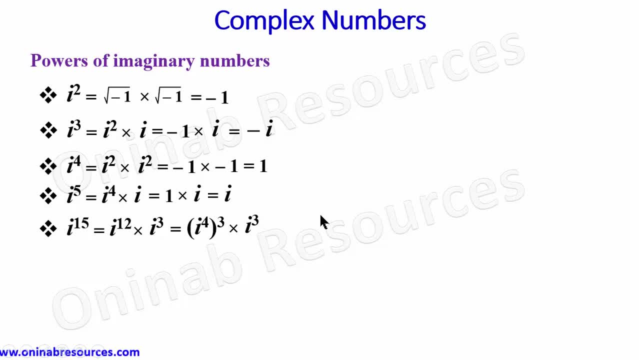 Then from here we know i raised to the power 4 is positive 1.. Then we now have it as i raised to the power 3, then times negative i, Since i raised to the power 3 is negative. so 1 raised to the power 3 is negative i. 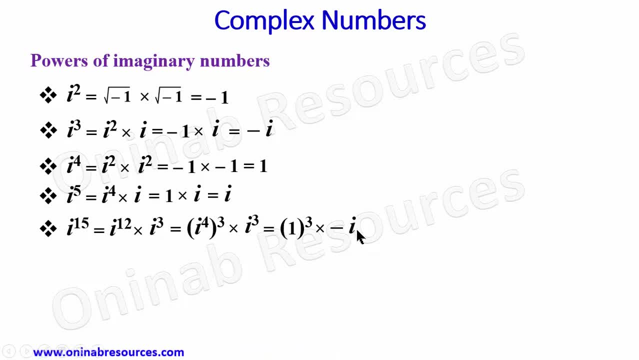 So 1 raised to the power 3 is 1.. Multiply by negative i gives negative i. Then for our information we can now look at it from the general point of view That in general for power n, where n is greater than 4.. 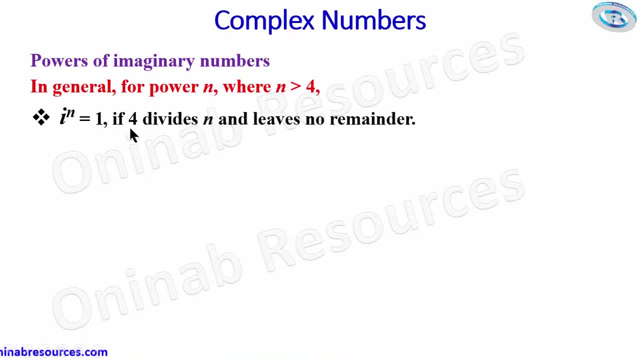 i raised to the power, n is equal to 1.. If 4 divides n and leaves no remainder, Okay, Like we saw in, i raised to the power 4, or we have it as i raised to the power 12.. Since 12 divided by 4 gives 3 without remainder, 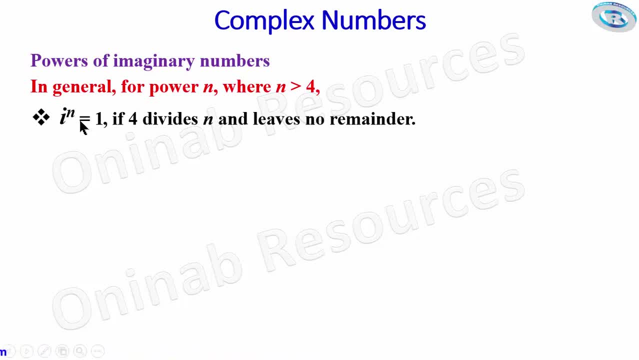 What we just do is we have i raised to the power 12 to be equal to 1.. Then also, i raised to the power, n is equal to i If 4 divides n and leaves a remainder of 1.. Can only leave a remainder of 0,, 1,, 2 and 3.. 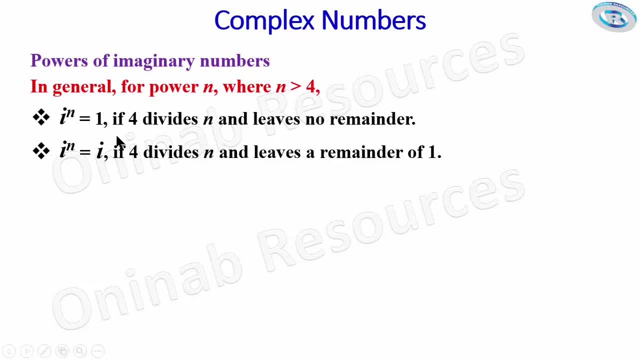 It cannot leave a remainder of 4.. So if 4 divides n and leaves a remainder of 1. Then i raised to the power n is i, Then also i raised to the power n is equal to negative 1.. If 4 divides n and leaves a remainder of 1.. 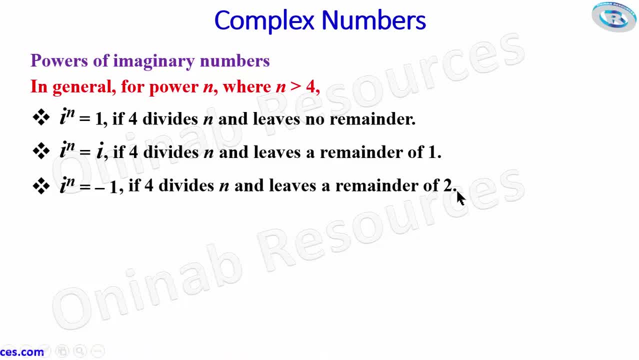 Then i raised to the power n is i. Then also, i raised to the power n is equal to negative 1. And i raised to the power n is i The remainder of 2.. For your information, you see, remember, I raised to power 2 is negative 1.. 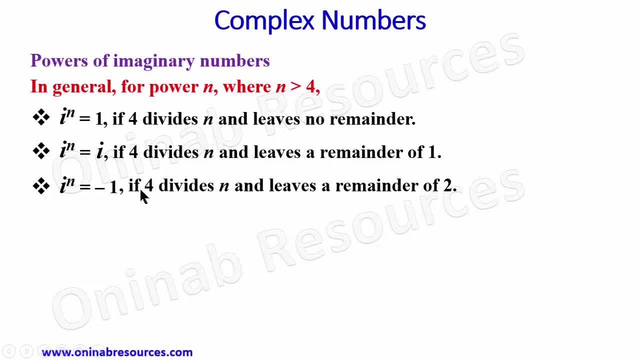 Okay, i raised to the power 2 is negative 1, since the i, the quotient, will always multiply 4 to give you a positive 1.. Then multiplying it by whatever power of i, that is the render, since i raised to power 2 is negative 1, then multiplying it by 1 with c, give us negative 1. 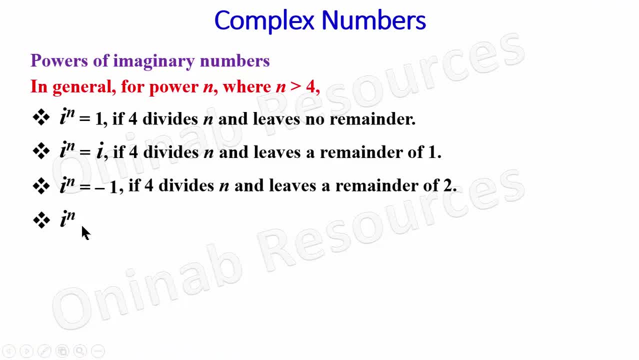 and lastly, i raised to power n is equal to negative i. if 4 divides n and leaves a remainder of 3, we saw that i raised to power 3 is equal to negative i from our previous slide. so the quotient times 4 to the power of i will always give us positive 1. so it is this remainder now. 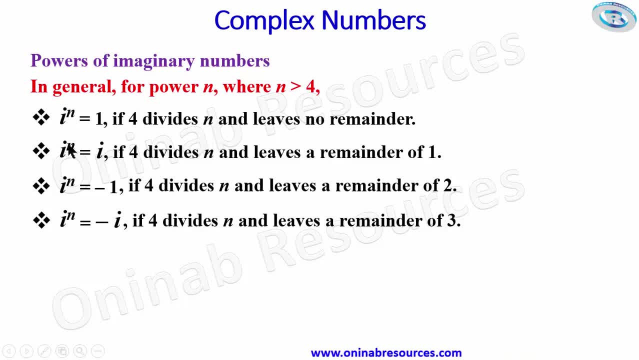 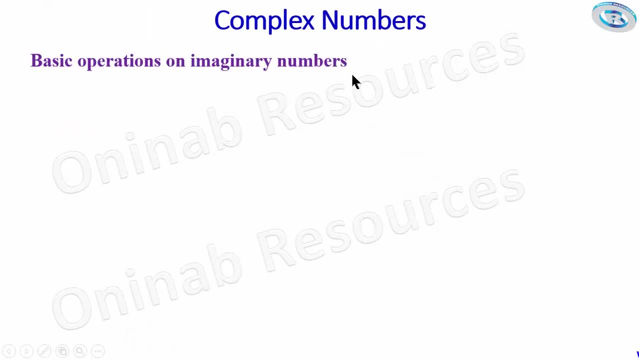 that will now determine the value of i raised to power n. so that is it for powers of imaginary numbers. then we now look at some basic operations on imaginary numbers. then here we go. evaluate imaginary numbers, each of the following: a- 2i plus 4i, b, 3i minus 7i, c 5i times 2i and d- 15i divided by 3i. 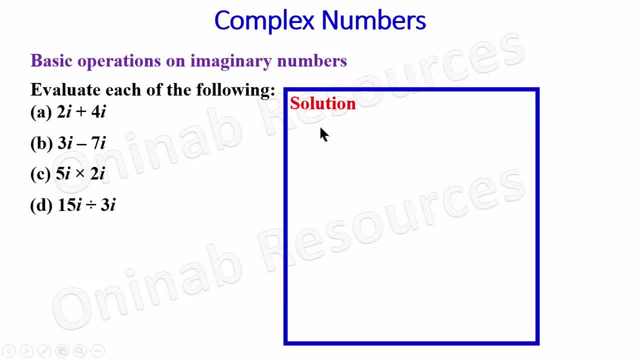 so in our solution we start from a, a 2i plus 4i, and that's going to just give us 6i. it is as good as saying 2x plus 4x, which gives 6x. so the same thing here: 2i. 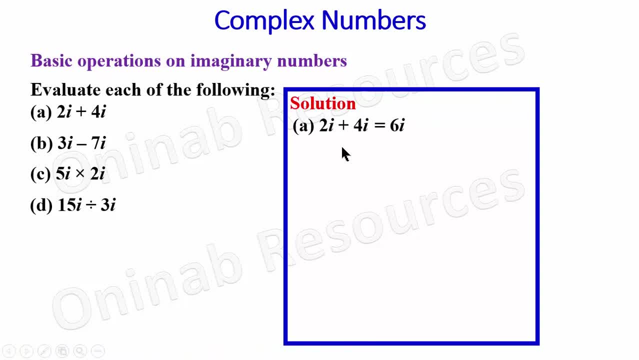 plus 4i gives 6i. then for b we have 3i minus 7i. 3i minus 7i, 3 minus 7, gives negative 4. so 3i minus 7i gives negative 4i. then for c we have 5i times 2i. so what we do here now is collect the coefficient. 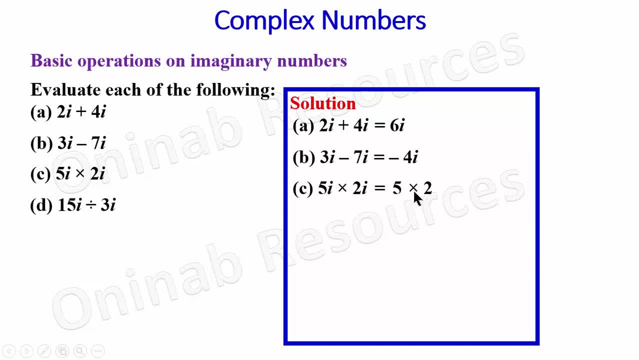 of the i's. that's 5 times 2i. so we have 5i times 2i. so we have 5i times 2i, so we have 5i times 2i times 2. 5 times 2 gives 10. then we now have i times i. so since 5 times 2 gives 10 and i times i. 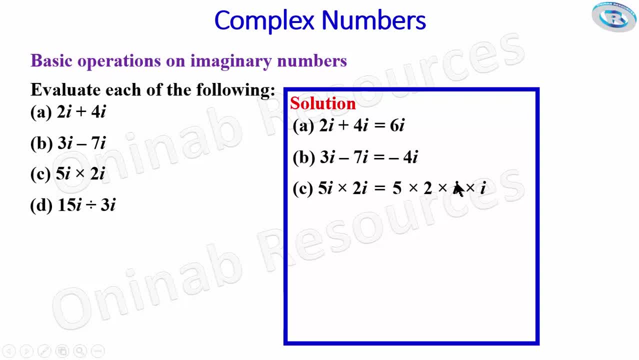 gives negative 1. so 10 times negative 1 gives negative 10. then we go for d. 15i divided by 3i is just going to give us 5. you know why it is 5? because we have 15 divided by 3i and we have 5i. 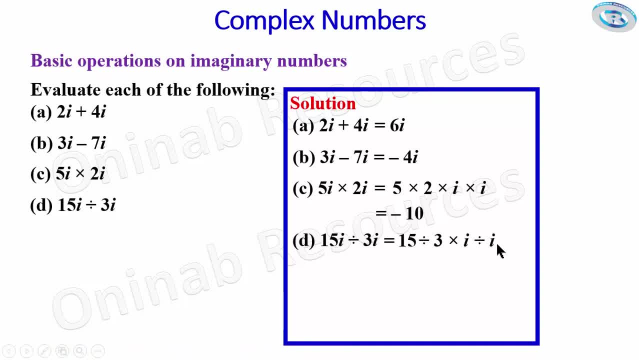 then times i divide by i, 15 divided by 3 is 5, and i divide by i gives 1, so we have our final answer as 5. so this is the highest we can take on basic operations on imaginary numbers and any other value. we follow the same pattern. we now go to basic operations on 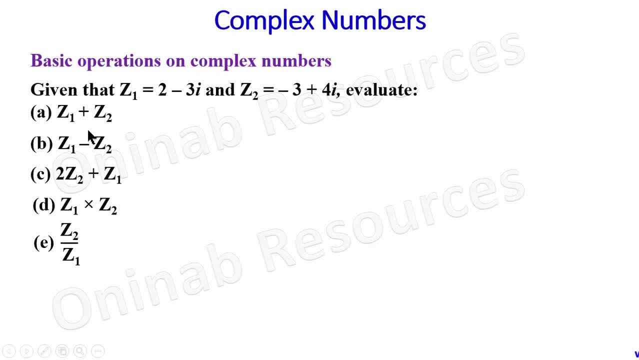 llamado coma, so that's also subtraction of complex numbers: c, 2, z plus z, 1. this is scalar multiplication of e, e, e, x. so this studies g, Lq. so inside out we have a function called E and from the equation let's see how this works. so let's say the complex number, the complex one, weekend. which is equal to z, has two is equal to zero. so Client e and X, so z 1, and I have e, e, e, e, and this times so e and z plus Zoom comes out Yo, because it is Milky theあ and for example, 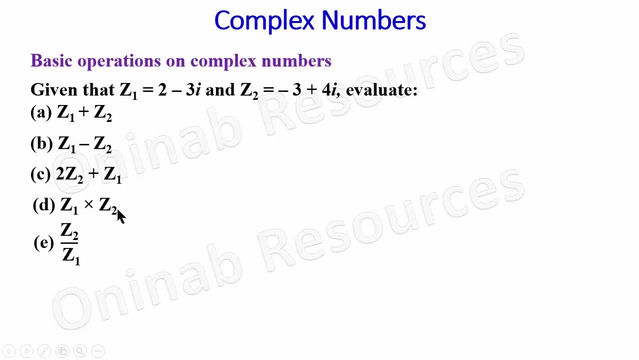 complex numbers: d z1 times z2, multiplication of complex numbers. and e, z2 over z1. this is division of complex numbers. so we start the solution of the problems from our solution. we start from a for a, we have z1 plus z2, so we can carry out our addition in a tabular form. it could. 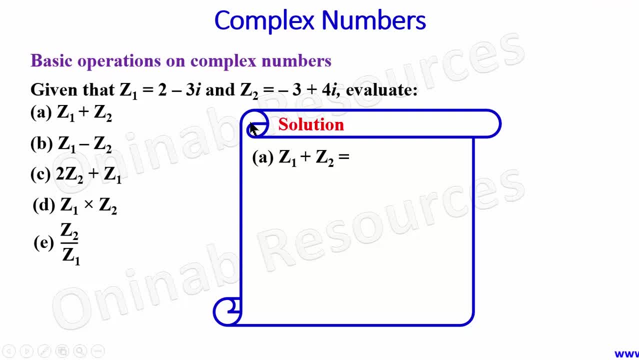 be multiplication in the tabular form. so z1 is 2 minus 3i, so I have 2 minus 3i, then plus z2, which is negative, 3 plus 4i. we then add in a tabular form: so, starting from here, 2 plus 3i. so what we? 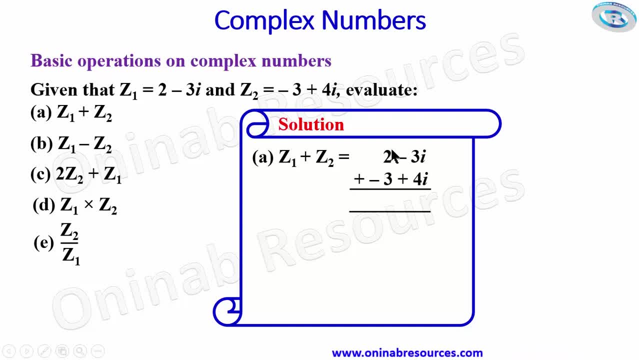 do here in our addition, we add the real parts and also add the real fibers. so we add the real fibers, so we get the real parts, like I said, so we get the real fibers and all we do here in our addition. we add the real parts and all. 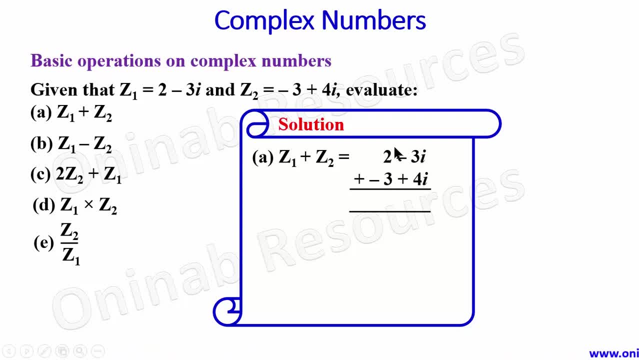 add the imaginary part. so we have for the real part is 2 plus negative 3. remember positive times negative is negative. so 2 plus negative 3 is 2 minus 3, which gives negative 1. then also we have a, the imaginary part, which is: 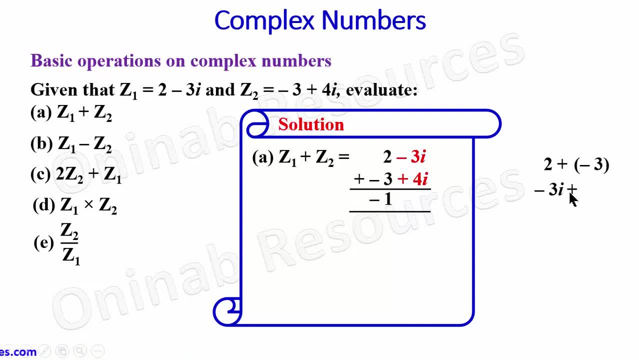 negative 3i plus 4. this is plus plus 4. that will give us plus 4. so negative 3 plus 4 gives 1. so we have our answer there as plus i. that's the end of solution to the addition of z1 and z2. then we go to B. so for B we have z1. 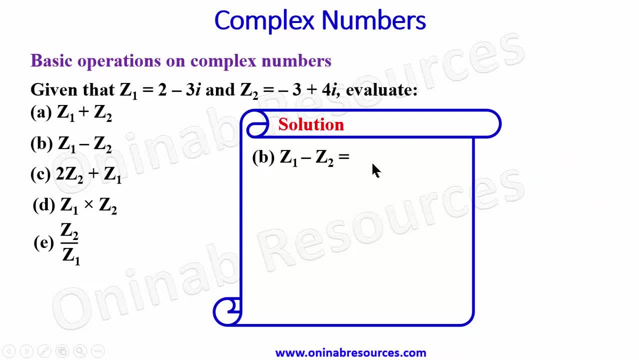 minus z2. also, arranging the subtraction in a tabular form, we have two minus three, i minus negative three plus four, i. again we are going to subtract the real part and thereafter the imaginary part. so from here we have the real part to be 2 and negative 3, so there are 2 minus negative 3 here, since negative times. 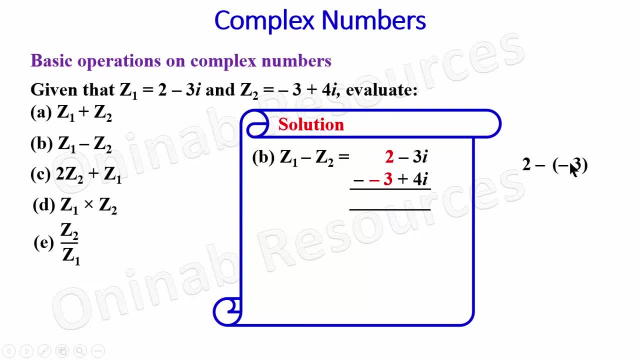 negative gives positive. 2 minus negative. 3 is the same as 2 plus 3, and that gives 5. then also we go to the imaginary part, so we have negative 3 minus positive 4, which is the same thing as minus 4. then we say minus 3i, minus 4i and that gives negative 7i. so we are done. subtracting. 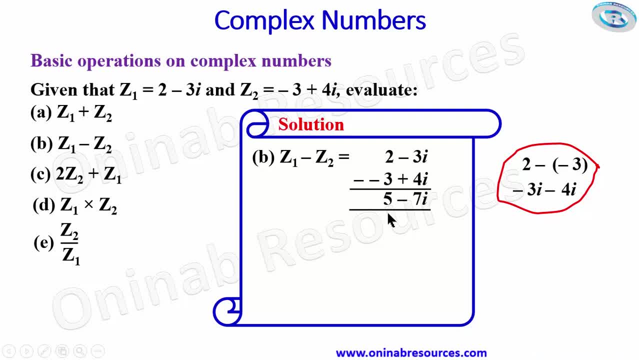 z2 from z1. then we go to the c part. for c we have 2z plus z1. first we simplify 2z2. um how do we do that? we just multiply z2 by 2. that's going to be 2 into negative 3 plus 4i. 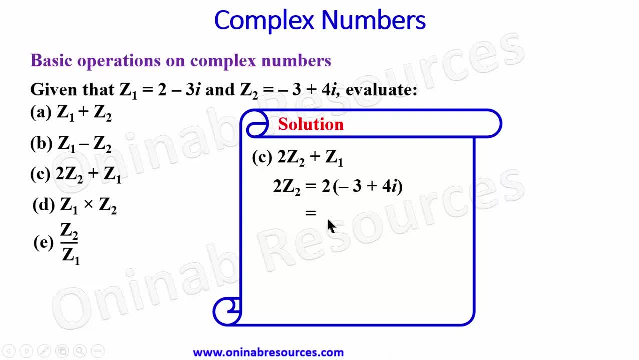 2 times negative 3 gives negative 6 and 2 times 4i gives positive 8i. then, going by our summation, now we have 2z2 plus z1, our 2z2 is negative, 6 plus 8i, then plus z1, which is 2 minus 3i. then we carry out the addition as we did in a 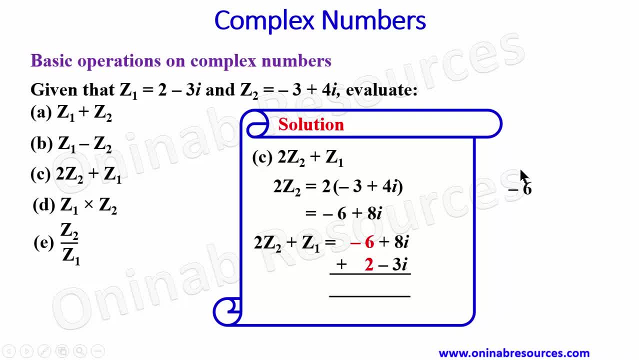 so the real part- that's going to give us negative 6 plus 2. negative 6 plus 2 will give negative 4. so we have negative 4 for the real part. then for the imaginary part, we have 8i plus negative 3i. so this is going to give us. 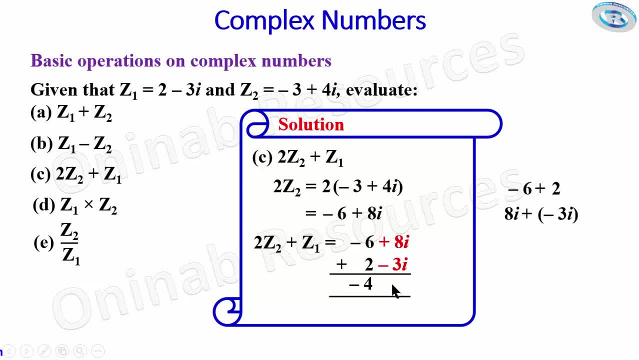 8i minus 3i, which gives plus 5i. and that is all for the c part of the problem. we go to the d part. so for d, this is multiplication: z1 multiply by z2, and that is going to give us z1, which is 2. 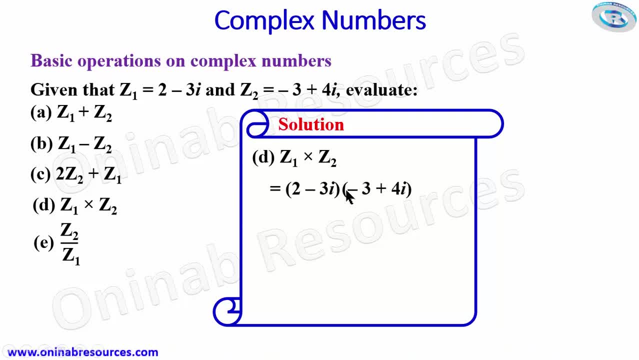 minus 3i in brackets, multiply by negative 3 plus 4i, which is the z2. this is just as good as the algebraic expansion that we know. so what we do is we pick this, the real part, and use it to multiply. multiply to mean remove 2i by the power of a-3.. now than we think to mean kill the AI uded as we want, but we think we also want to catch an AI model that we don't want to be taught. so we pick this isiana. this is the c part of the equation- and then we multiply this, and to do that we need to multiply it by m in smart en служ, but 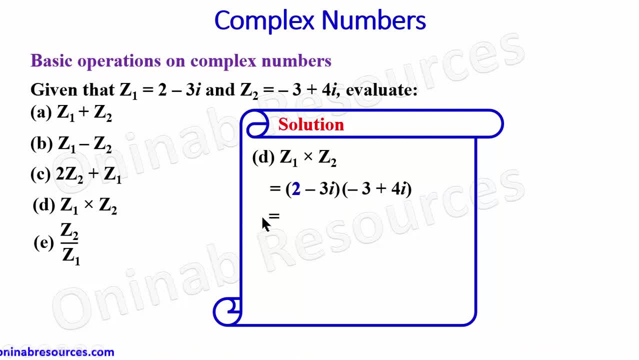 think of this as enforcement part in the second bracket. so we have it as 2 into negative 3 plus 4i. then thereafter we pick this, the imaginary part, we use it to multiply every part of the second bracket. so we have it as negative 3i into negative 3 plus 4i. then 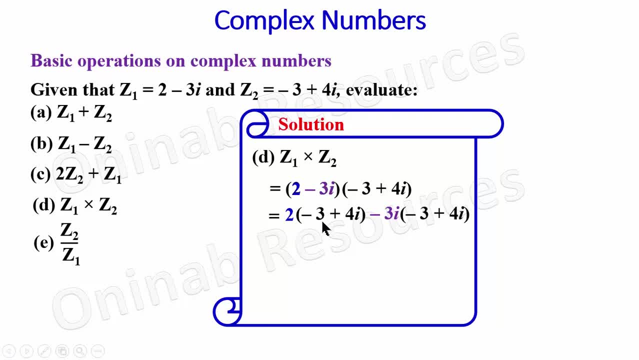 we expand and simplify: 2 times negative, 3 gives negative 6, and 2 times positive: 4i gives positive 8i. we are done with this part. then we go to the other part: negative 3i times negative, 3 gives positive 9i, then negative 3i times. 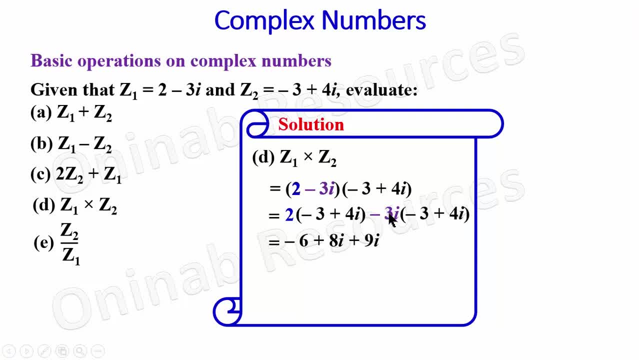 positive 4i. for your information, negative 3 times positive 4 gives negative 3i 12. then i times, i gives negative 1, so that negative 12 times negative 1 gives positive 12. then we simplify the real part and then the imaginary part. this is: 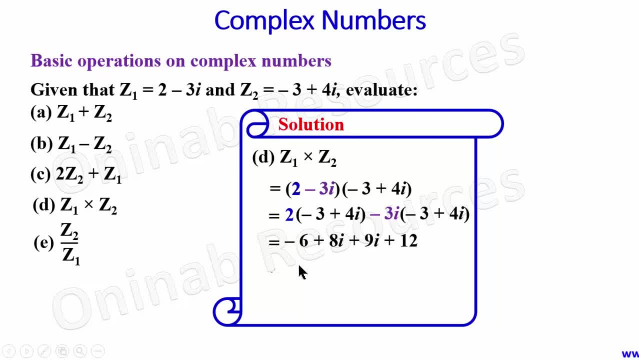 negative 6 plus 12 and that will give us a 6. then positive 8i plus 9i gives positive 17i. that's the end of solutions. solution to the product of z1 and z2. remember it could be written as z1, z2, so. 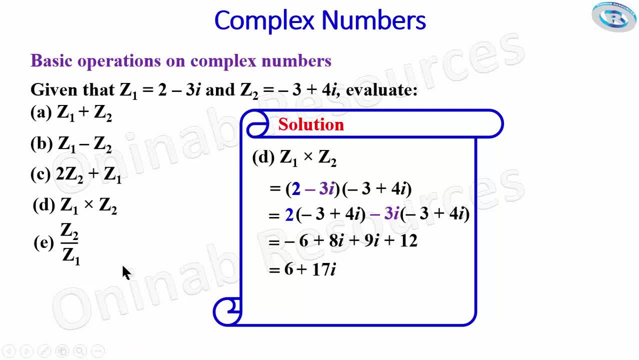 whatever you see there, it is going to be product. so we go to the e part of the problem. for e, we have z2 divided by z1, so we are going to have it as z2, which is negative. 3 plus 4i over 2 minus 3i. that's what we call. 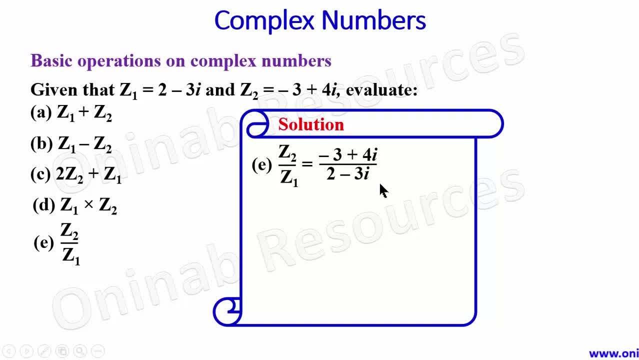 father ot. I don't want to do that first in instant process. the final. Thank you for watching this video today. we hope that you enjoyed this lesson by you until the end. so i will continue at noon as we go on. so the connector here is negative, so its conjugate will just be positive. So if the connector is, 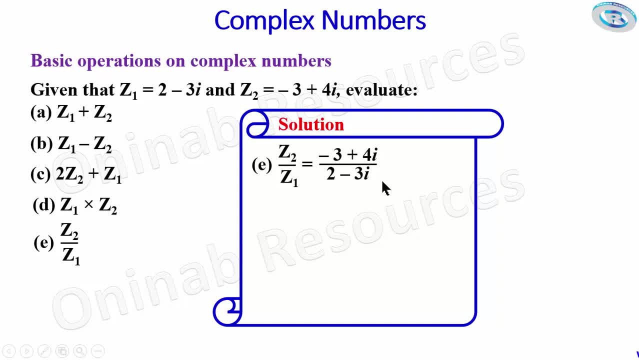 positive, its conjugate will just change to negative. Like for Z2, the conjugate of Z2 is going to be negative, 3 minus 4i, while the conjugate of Z1 is 2 plus 3i. So that is that for. 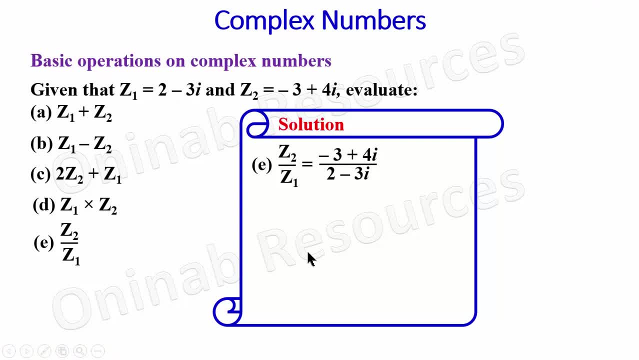 Z1 and Z2 conjugate. So, coming back to our problem, we are going to multiply the numerator by the conjugate, which is 2 plus 3i. So we have multiplied by 2 plus 3i over 2 plus 3i. 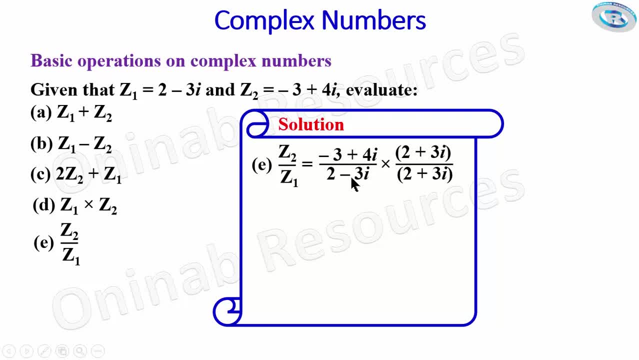 So, whatever you do to the numerator, you also do it to the denominator in order to balance everything, because this is as good as multiplying by 1. Which does not add any value to the expression. So, doing that, we have negative 3 plus 4i. 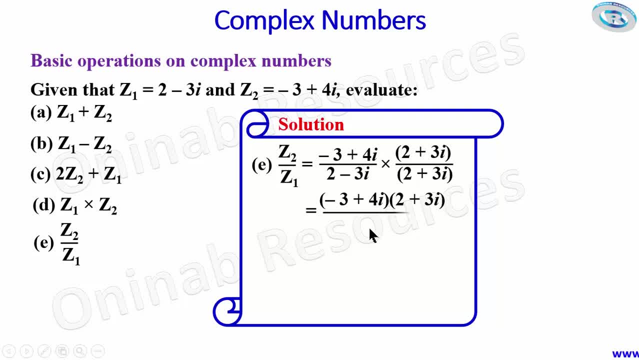 times 2 plus 3i over 2 minus 3i into 2 plus 3i. The expansion of the numerator is going to be like what we did in D. Why the expansion of the denominator? Because they are conjugates of each other. We just multiply the real part and the imaginary part. We then 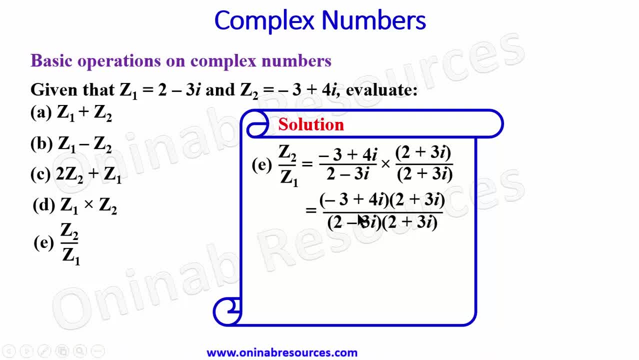 conclude that expansion. For the expansion of the numerator, I pick the first part, that is the real part in the first bracket and use it to multiply everything inside the second bracket so that we now have negative 3 times 2 gives negative 6, and negative 3 times positive 3i. 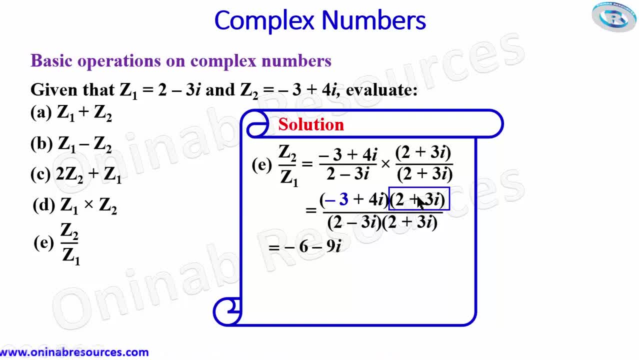 gives negative 9i. So we are done with that. We pick the second part of the first bracket, which is the imaginary part that is plus 4i. We use it to multiply everything inside the second bracket. So positive 4i times 2 will give us positive 8i. Positive 4i times positive: 3i- Remember- 4 times 3. 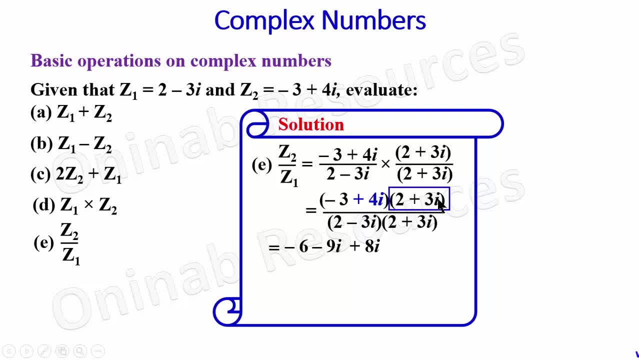 gives 12. And i times i gives negative 1.. So 12 times negative 1 gives negative 12.. Then over, What we are saying is for the expansion of the denominator. as we explained earlier, we multiply out the real part and then the imaginary part. We 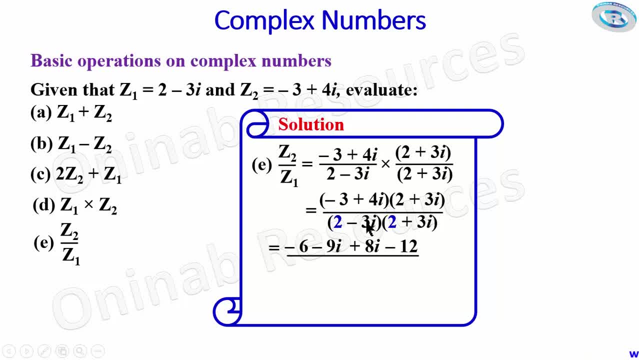 said, we are multiplying two by two and the imaginary part, which is negative, 3i times the positive, 3i. So we multiply out and simplify, So we have 2 times 2, which gives 4, and negative, 3i times positive, 3i Negative, 3 times negative, 3 gives negative, 9 and i times i. 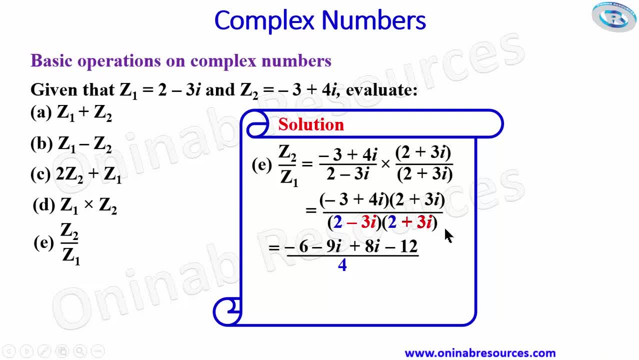 gives negative 1.. So negative 9 times negative 1 gives positive 9.. So we then simplify and have our final answer for the division of the complex numbers. So this is: negative 6 minus 12 gives negative 18 and negative 9i plus 8i gives negative. i then over 13.. And that's all for the 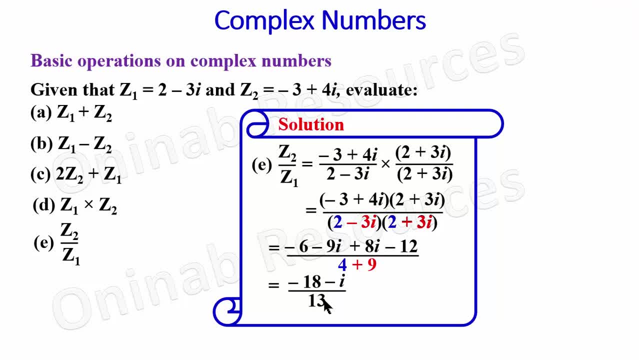 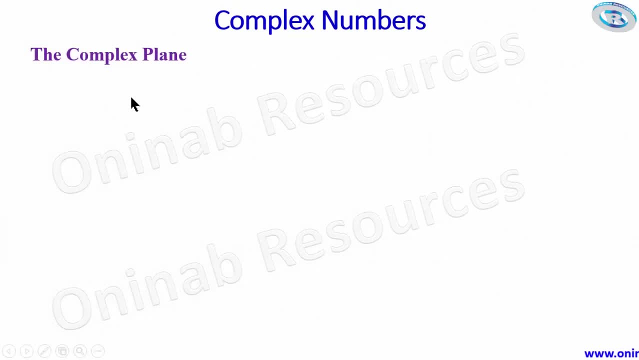 division of z2 by z1.. So we are done with basic operations on complex numbers. We then go to the complex plane. For the complex plane, we know our Cartesian plane is a plane of x and y axis. So in the knowledge of sabenow, we have broken it. So now we have broken from x, y and z2. so our 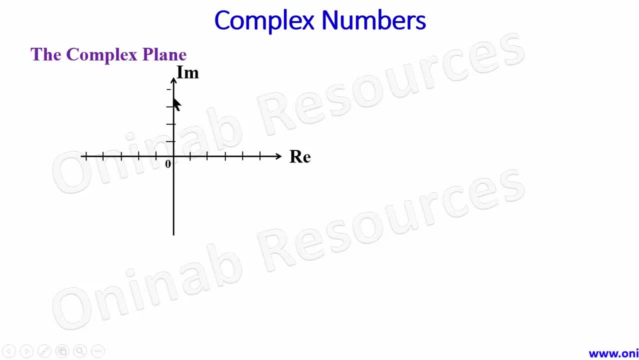 ∑z is a plane of zero and z2 is a plane of three. Of course, if we stay the same, weääare the original product. 1 unit here is going to be negative. 2 negative, 4- this is 2i, 4i, and here is negative 2i and negative. 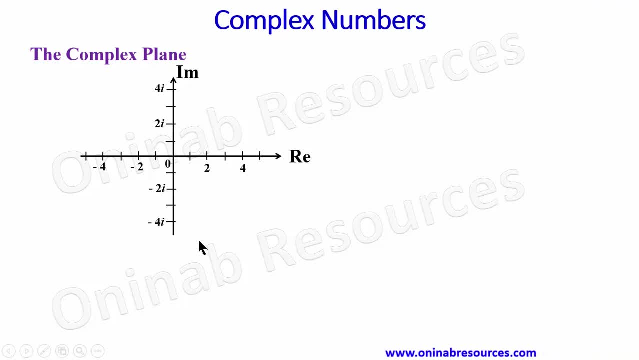 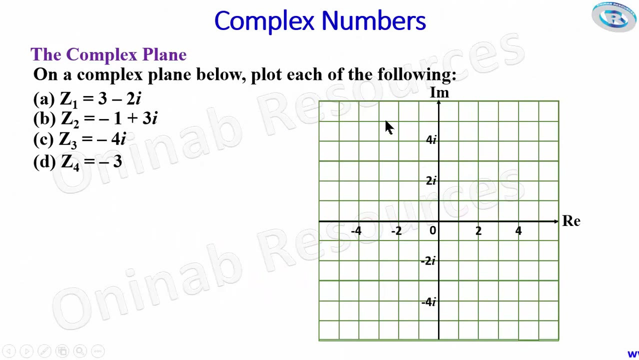 4i. this is the complex plane. so the next thing is: how do we plot the complex numbers on the complex plane? so we go here on a complex plane- below this is the complex plane plot, each of the following: we have z1 to be 3 minus 2i. we have z2 to be negative, 1 plus 3i, z3 to be negative, i and z4. 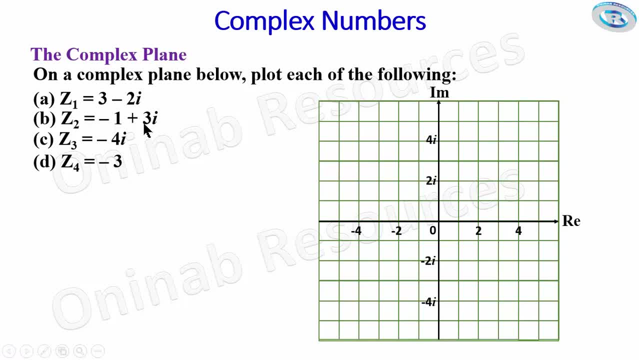 to be negative 3. starting from a, we have the real part to be 3 and the imaginary part to be negative 2i. so here, on the real part, this is 3. this is the line where the real part is 3. then for the imaginary part, we: 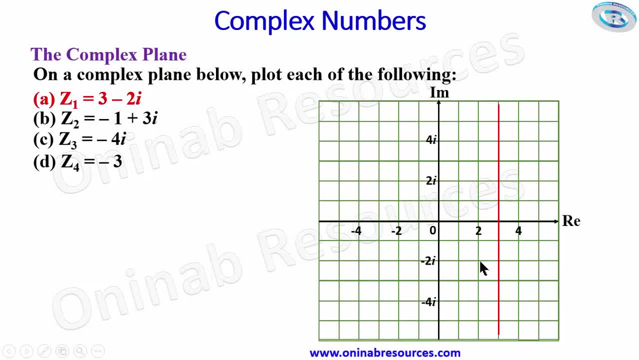 have negative 2i. here is the line where the imaginary part is negative. 3i. their point of intersection is this, and that will represent our z1. so that is the point for z1 on the complex plane. then for z2, that is the b, the real part is negative 1. this is the line where the real part is negative. 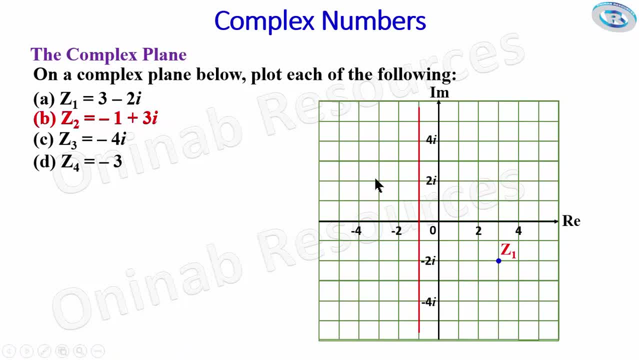 1 and the imaginary part is positive 3. this is the line. the imaginary part is positive 3.. their point of intersection is here, so we label that point as z2. so that is the z2 on the complex plane. then for z3, the real part here is zero. the z3 can be written as zero minus 4i, where the real part is zero, and